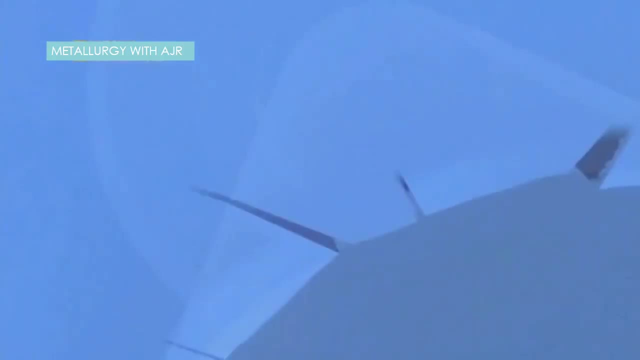 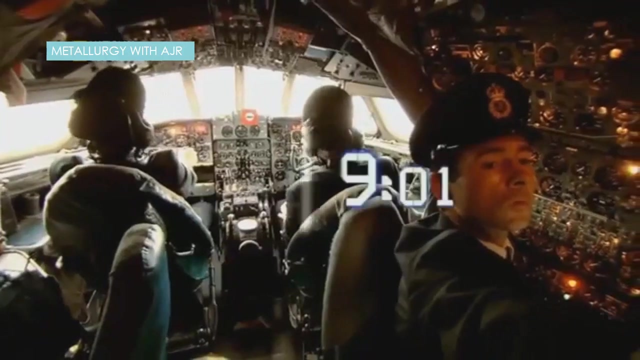 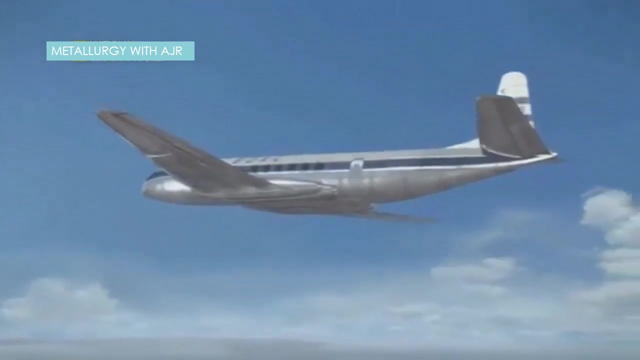 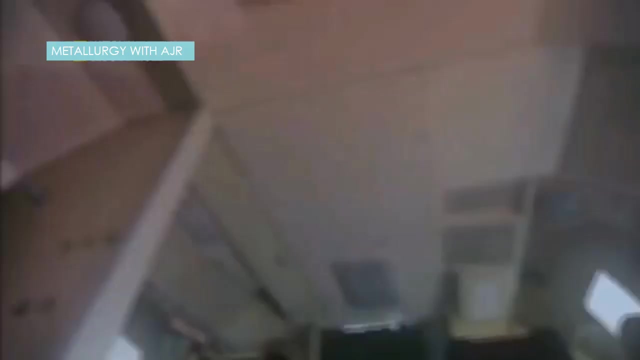 This odds which gave the fracture to start. So cracks can appear in diverse types of structures, such as planes, boats, brichorg cranes, overhead cranes, and either on rail away access. The discovery of fatigue occurred in 1800, when several investigators in Europe observed that bridge and rail components were cracking when subjected to repeated loading. 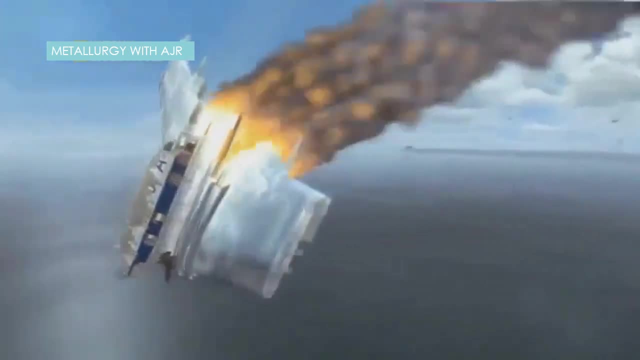 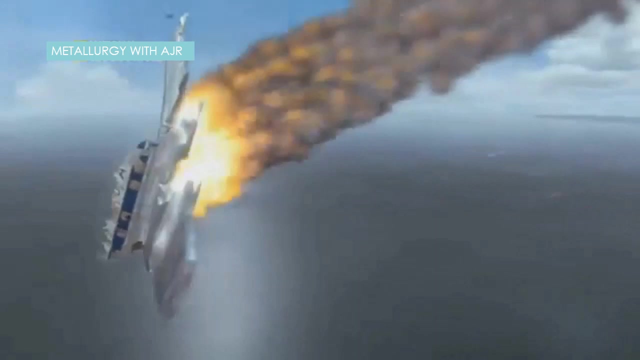 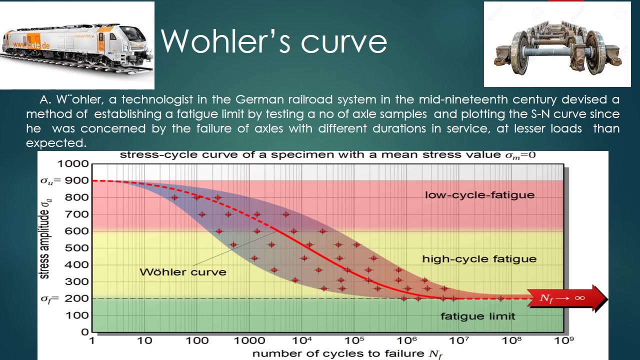 use of metals expanded. with increasing use of machines, more and more failure of components subjected to repeated loads were recorded. Wohler proposed a method by which a failure of components from repeated loads could be solved. As already stated Wohler, a technologist in the German railroad system, in the mid. 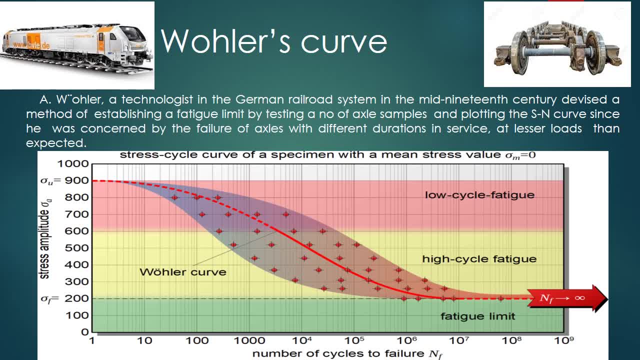 19th century, devised a method of establishing a fatigue limit by testing a number of axle samples and plotting the SN curve, since he was concerned by the failure of axles with different duration in service at lesser loads than expected. You can see the SN curve here, the stress versus number of cycles First. 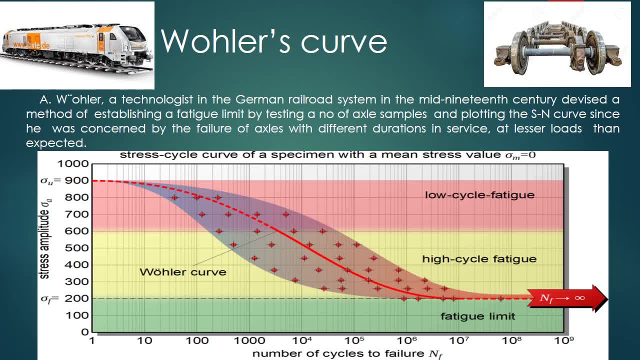 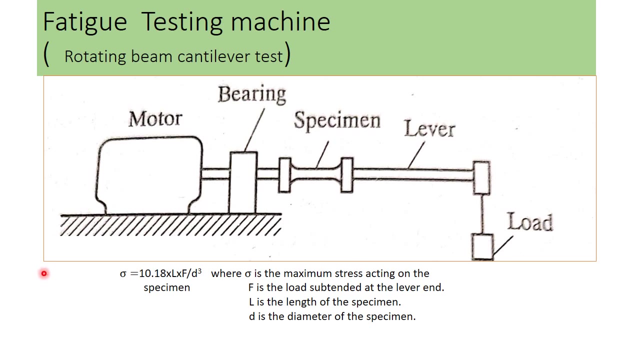 the curve, it decreases exponentially and moves to a steady state. that steady state is defined as the fatigue limit. Here, at stress level below the fatigue limit, the axle will indefinitely work. A common method to measure the resistance to fatigue is the rotating beam. cantilever test A weight. 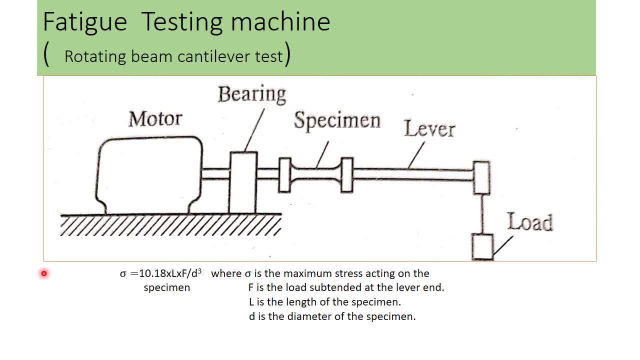 presented from the one end of the tensile specimen. as shown in the figure, The specimen initially has a tensile force acting on the top and the bottom surface is compressed. then, when the specimen turns another 90 degree, the location that were originally in tension and compression have no stress acting on. 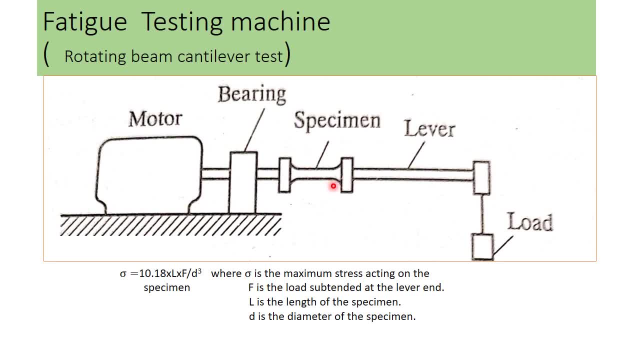 them. After a half a revolution of one 8o degree, the material that was originally in tension is now in compression. thus the stress at any point goes through a complete cycle: from zero stress to maximum tensile stress, to zero stress to maximum compressive stress, the maximum stress. 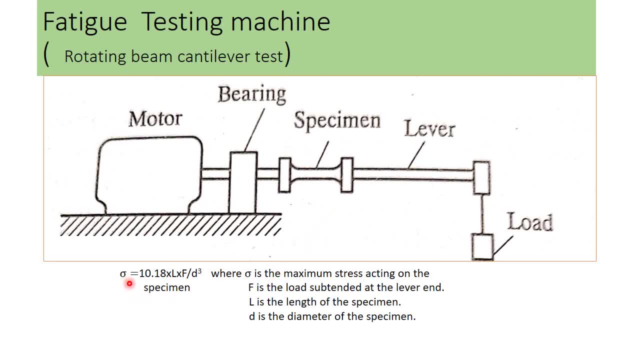 acting on the specimen is given by this formula: sigma is equal to 10.18 into le, into f divided by dq, where sigma is the maximum stress acting on the specimen, f is the load subjected at the lever end and l is the length of the specimen and d is the diameter of the specimen. 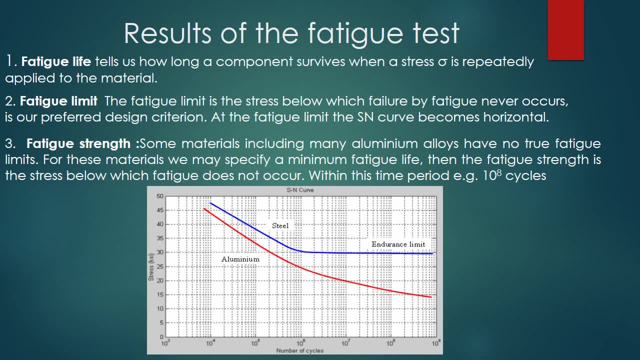 the results of the fatigue test. fatigue life tells us how long a component survives when a stress sigma is repeated to the maximum stress acting on the specimen. the results of the fatigue test. fatigue life tells us how long a component survives when a stress applied to the material fatigue limit. fatigue limit is the stress below which failure by fatigue. 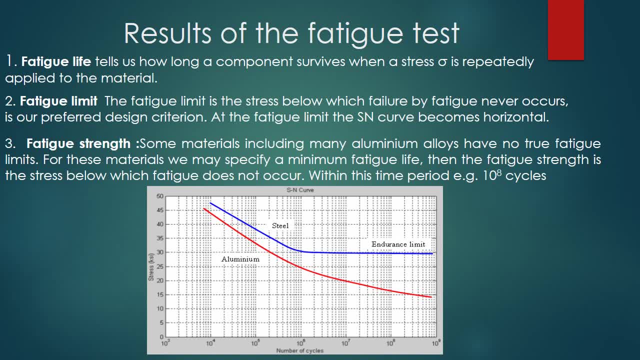 never occurs is our preferred design criteria. at the fatigue limited, the s? n curve becomes horizontal. this is only in the case of steel. in steel you can see a perfect fatigue limit. it is also called endurance limit. so below this limit the stress is always in the case of steel and it is considered to be a very important factor. 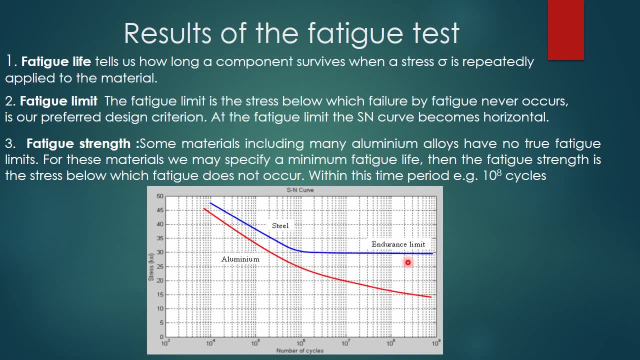 in the case of steel, it is considered to be the most important factor in the development of the human body and in this way the component can survive an indefinite number of cycles. fatigue strength: fatigue strength is applicable only for aluminum alloys, because in aluminum alloys you are having a exponential decrease and the curve is always in exponentially decreasing. 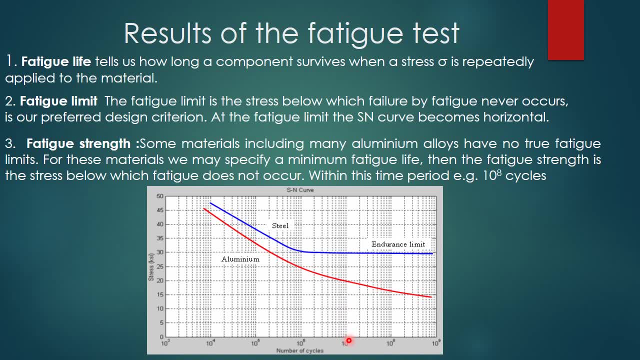 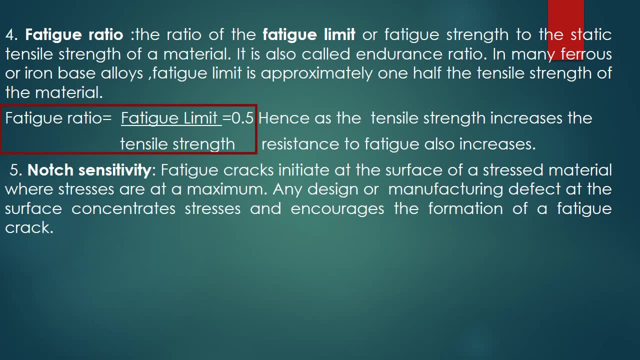 at 10 power, 7 cycles like that we are defining the fatigue strength. for our design purpose we need a very important parameter called fatigue ratio. fatigue ratio is the ratio of fatigue limit by tensile strength. we know very well the tensile strength of the material so we can calculate the fatigue limit. since the 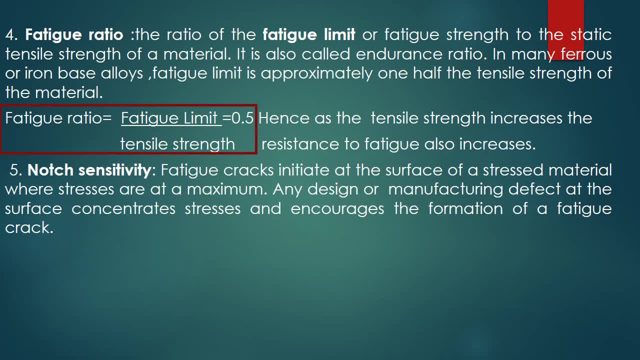 fatigue ratio is equal to 0.5. the next is not sensitivity. fatigue cracks initiated the surface of a stressed material where stresses are at a maximum. any design or manufacturing defect, like change of cross-section at the surface, concentrates stresses and increases the formation of a fatigue crack. 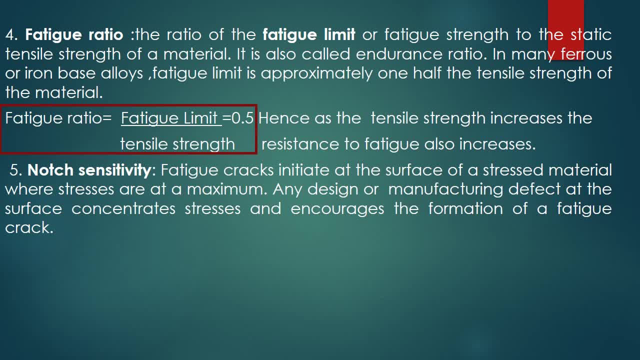 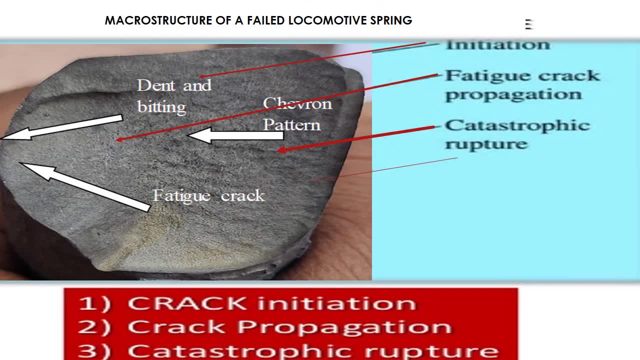 this is more pronounced in rainfall access where change of cross-sections are very, very prominent. this is the macro structure of a failed locomotive spring. for better understanding of the failure mode and factor graphic, we are just examining the factor graph he of a failed locomotive string. intent is: 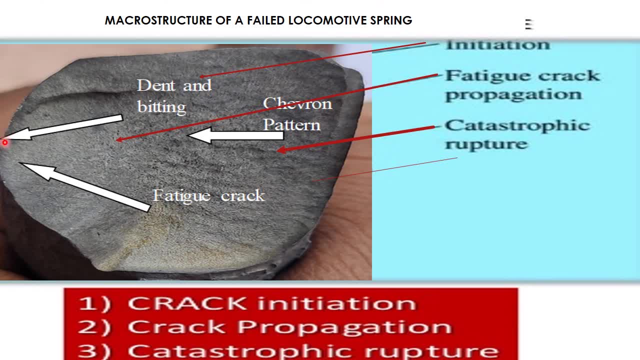 present at the extreme end of the tractograph, that is, on the surface of the spring, and from the dent the fatigue crack starts propagating. here, finely spaced lines you can see. they are called beach marks. they are very closely spaced because when they are closely spaced it means that the fatigue crack is propagating very. 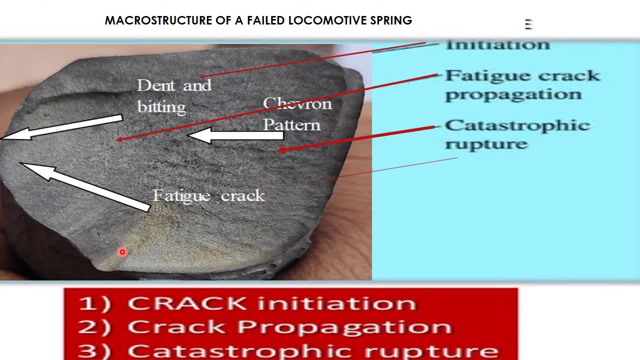 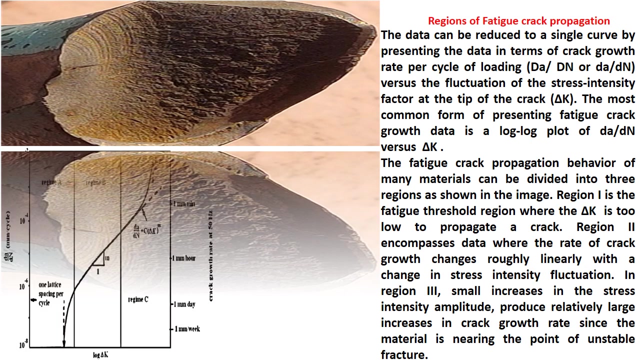 slowly, one day and after a particular time, you can see the fatigue crack has covered up to this particular portion. and the third, final part is the catastrophic rupture. the catastrophic rupture is characterized by the chivron pattern: fatigue crack propagation here dnr by dnr is the crack growth rate per cycle of loading and delta k is the stress. 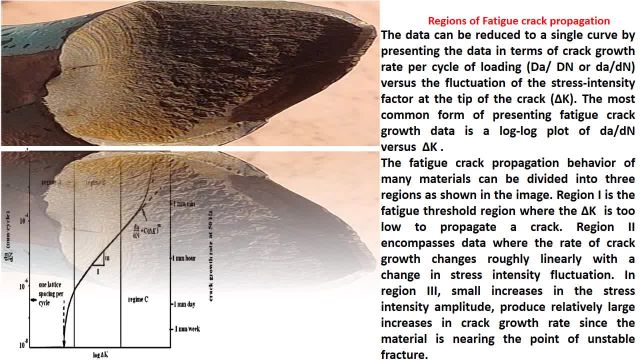 intensity factor at the tip of the crack. the most common form of presenting the fatigue crack growth data is a log log plot of da by dn versus delta k. here you can see the fatigue crack propagation. the macro structure is presented at the top portion and here the curve is given.